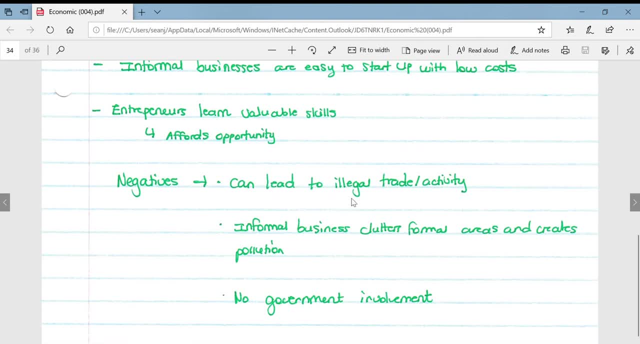 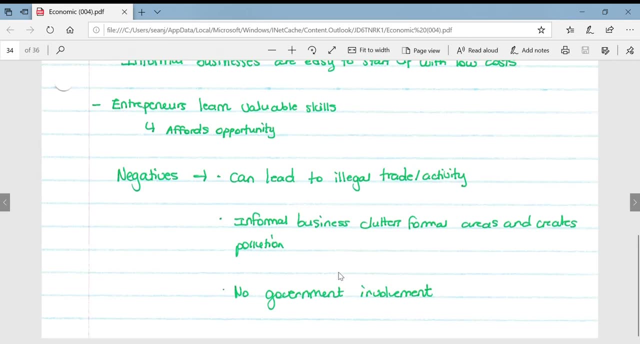 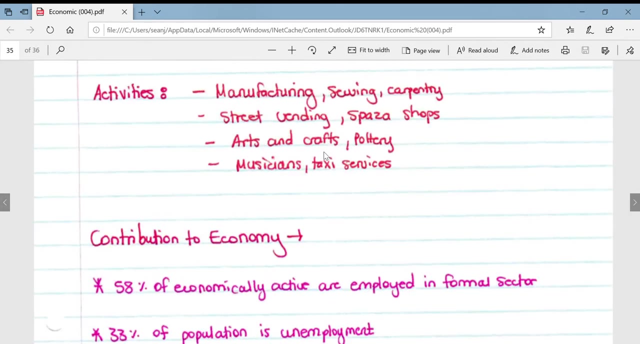 Some of the negatives of the informal sector can lead to illegal trading or activities. Informal businesses clutters the formal areas and creates pollution. There's also very limited government involvement. The main manufacture are the main activities within the informal sector: Manufacturing: sewing. 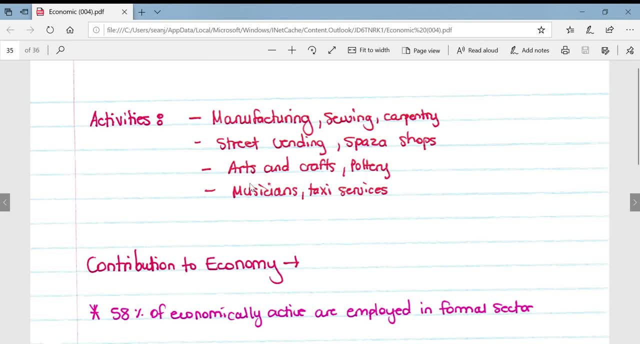 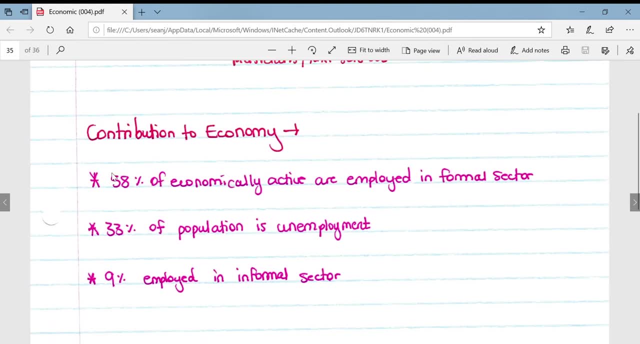 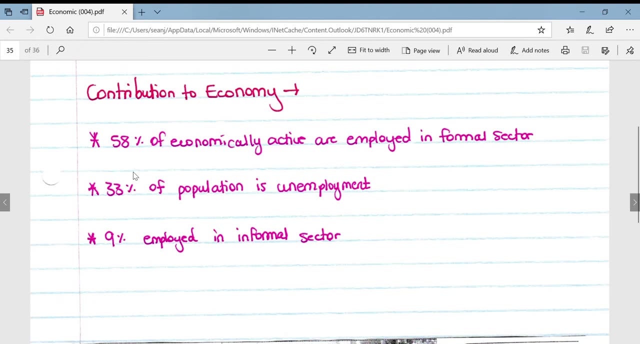 carpentry street, vending spaza shops, arts and crafts such as pottery, musicians and taxi services. Contribution to the economy: 58% of the economically active portion of the population are employed in the formal sector, 33% of the population is unemployed and 9% are employed in the informal. 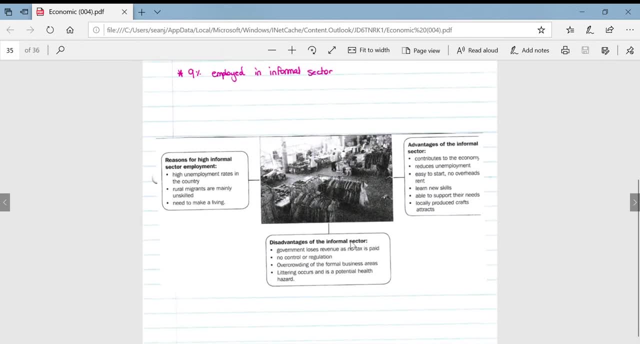 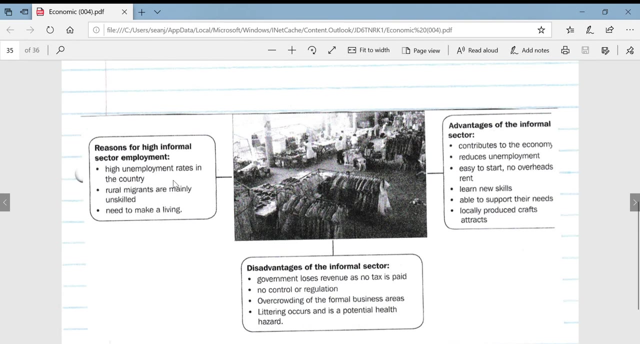 sector, Then if we just look at this little mind map, I give credit to the geography study guide. I highly recommend this book to use in addition to these videos. Reasons for high informal sector employment. High unemployment rates in South Africa. Rural migrants are mainly unskilled need to make a living. Disadvantages of the informal sector: Government loses revenue as. 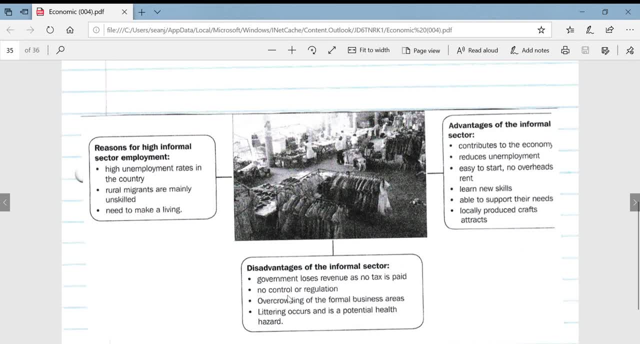 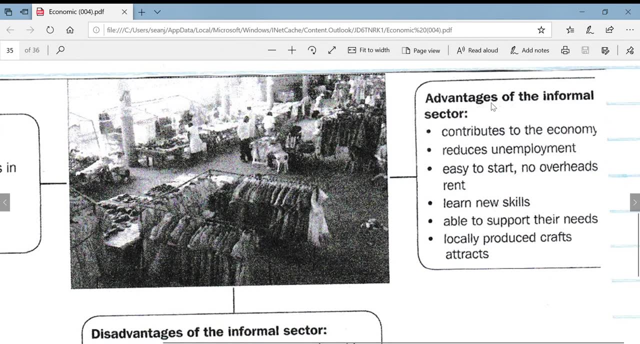 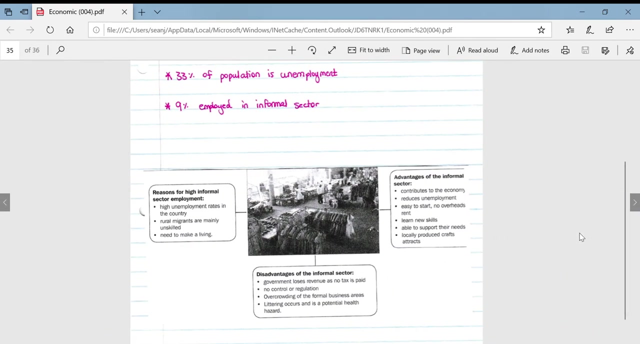 no taxes paid, no control or regulation, Overcrowding of the formal business areas and littering occurs and is a potential health hazard. Overcrowding of the formal business areas and littering occurs and is a potential health hazard. Then the advantages of the informal sector: contributes to the economy, reduces unemployment, easy to start with no overheads, rent, learn new skills, able to support people's needs and locally produced crafts, attracts many tourists, etc. 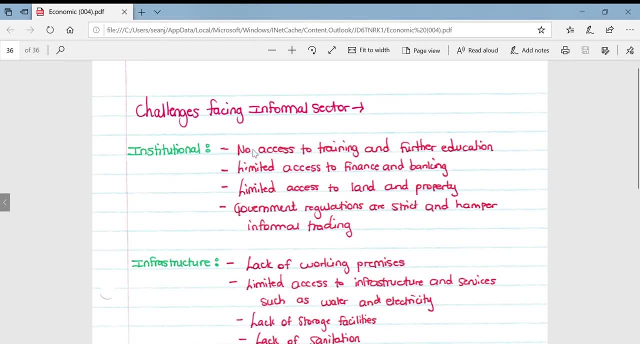 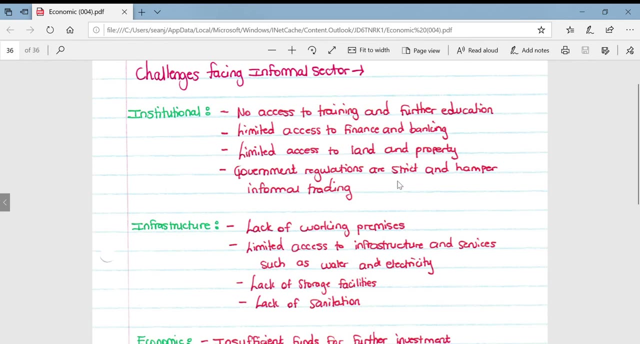 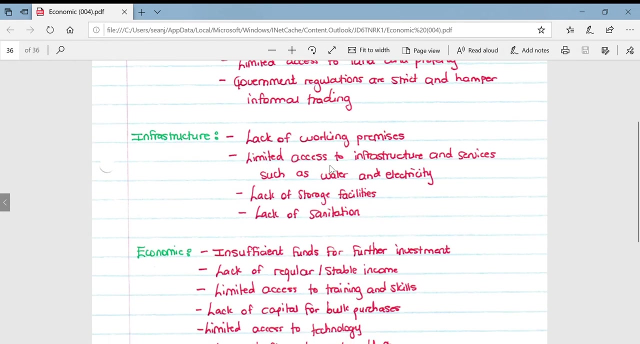 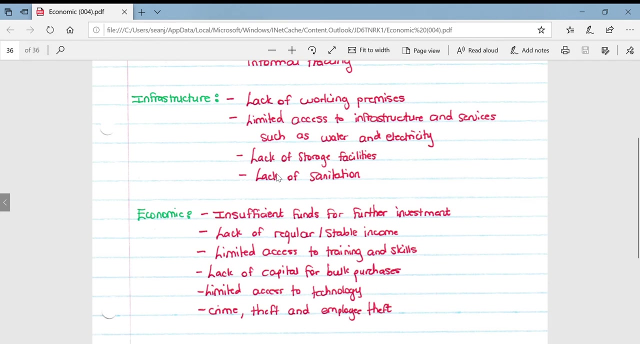 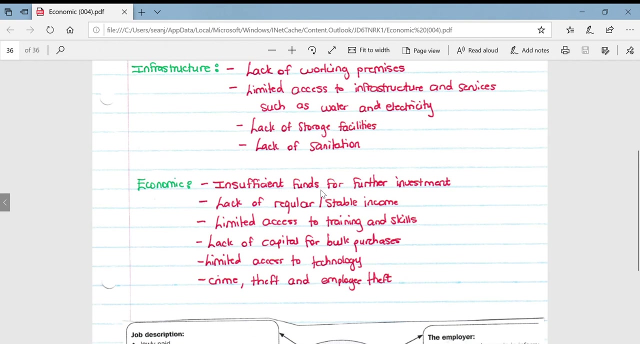 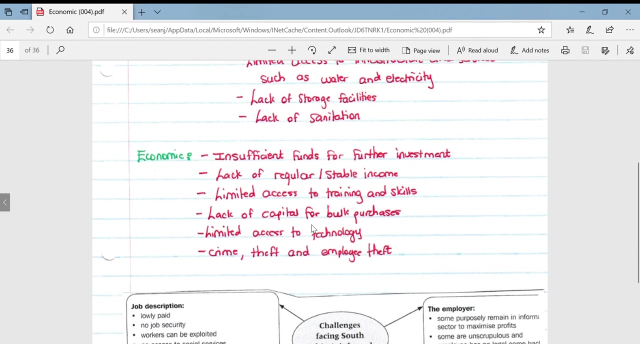 Then some of the challenges facing the informal sector of storage facilities and lack of sanitation, and if we look at some of the economic challenges associated with the sector: insufficient funds for further investment, lack of regular, stable income, limited access to training and skills and a lack of capital for